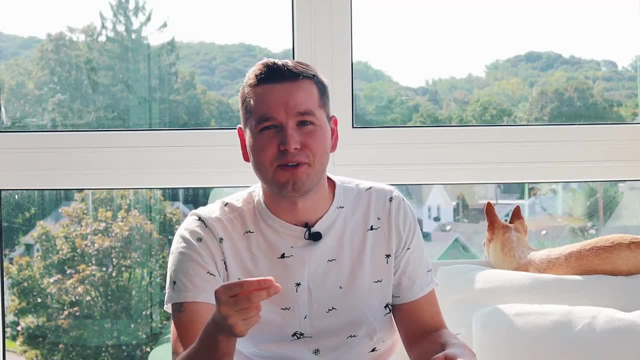 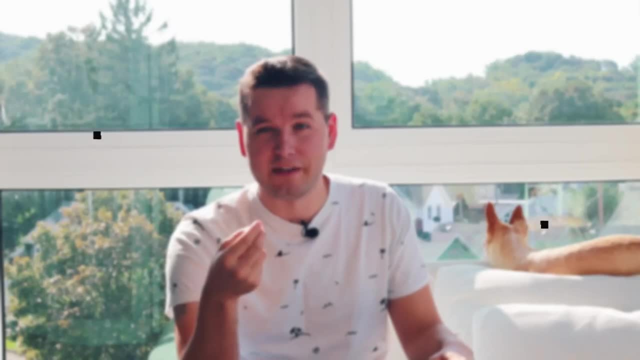 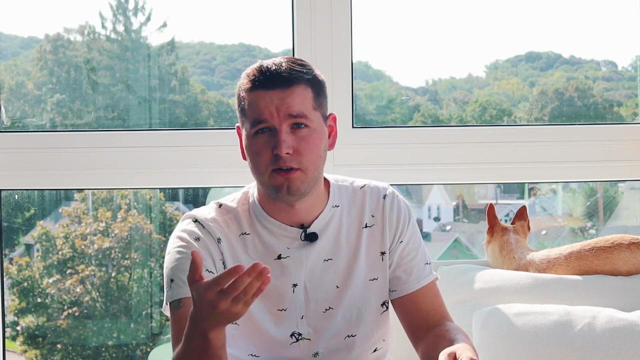 Since C has been around for so long, it has actually served as the foundation for many programming languages, just as I mentioned. Because of that, it has also served as the foundation of the syntax for other programming languages. It might be easier for you to read those languages or actually learn those languages. 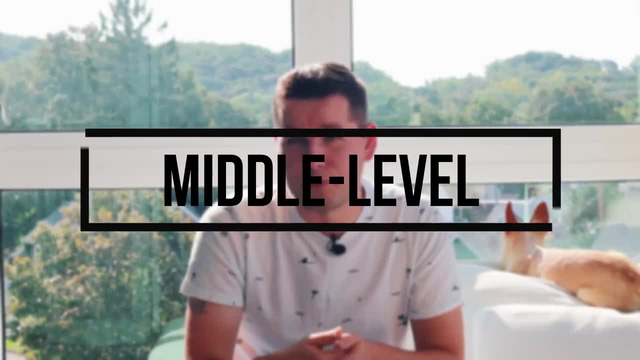 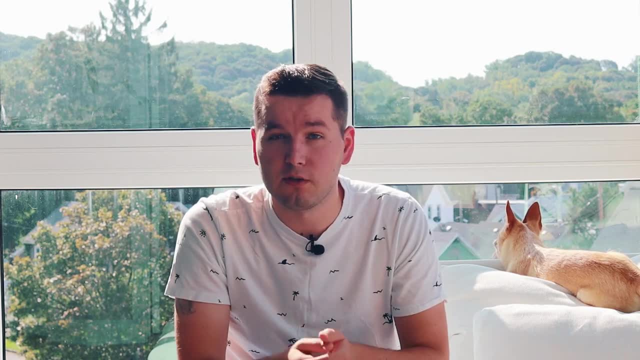 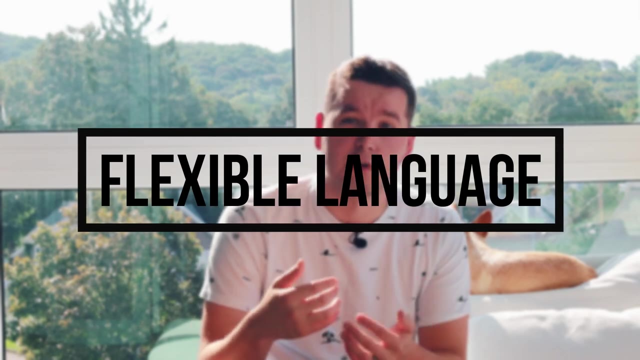 because you already know something about C programming. It's a middle-level programming language that supports both high and low-level programming. Thus it can closely work with the registers of the CPU to write some drivers or actually write some applications on the higher level. It's also a flexible language that can run on different compilers and on most hardware. 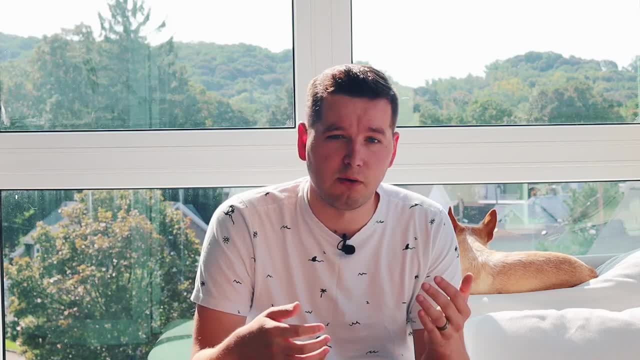 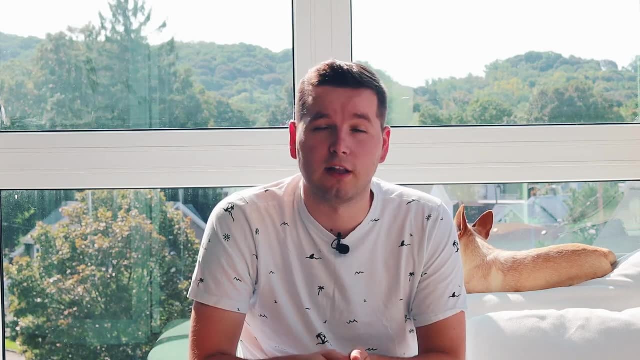 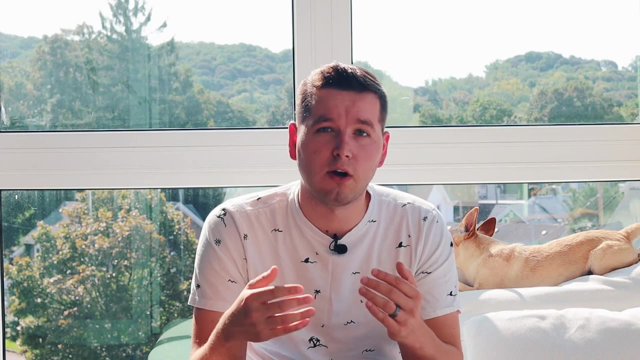 meaning you could write code on your Windows computer and then go on a Mac OS and just still run that code without any issues. Also, most microcontrollers support C as a programming language to program them. Dynamic memory allocation- meaning you can allocate memory during runtime. in C, For example, you can use calls for memory allocation to change the size. 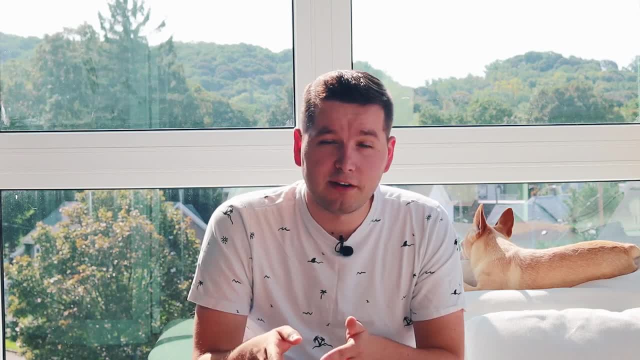 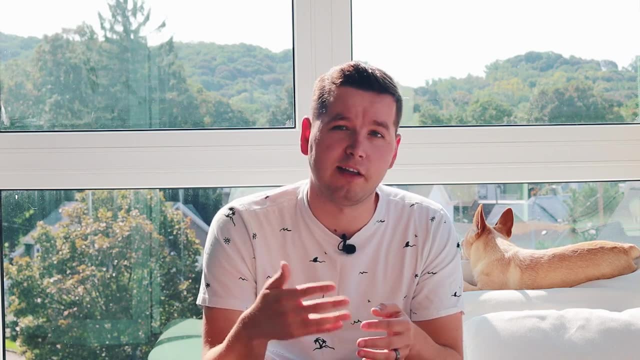 of an array while the code is running, Although in embedded environments you do want to be careful with doing that, just because you have limited amount of memory, so you want to keep that constraint in mind. Last pro is it can implement algorithms and data structures fast, Being a 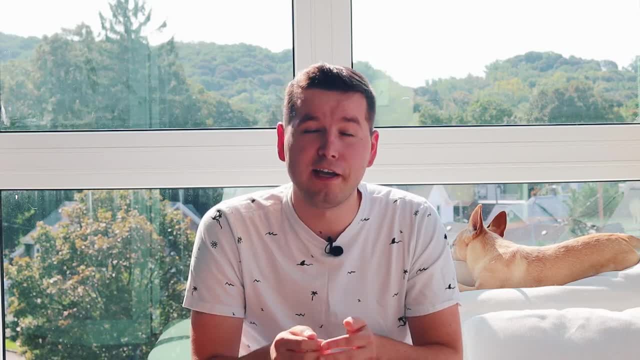 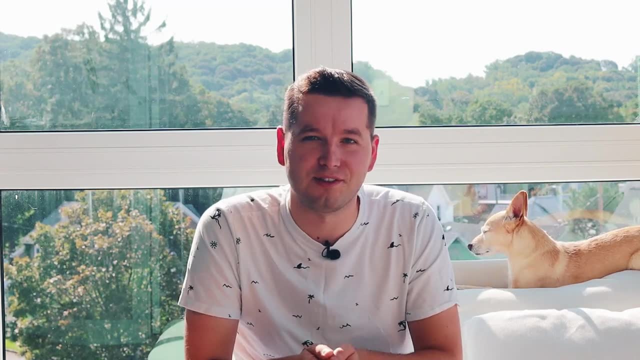 able to perform and calculate complex algorithms fast is pretty important for embedded development. Well, those are the pros of learning C for embedded software engineering. Now let's move on to the cons. The biggest con is that if you haven't subscribed to my channel yet, consider doing it. 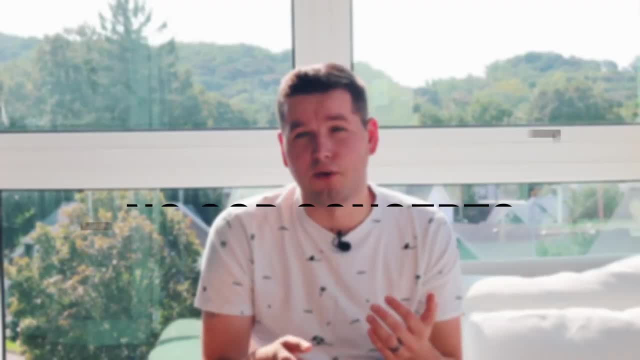 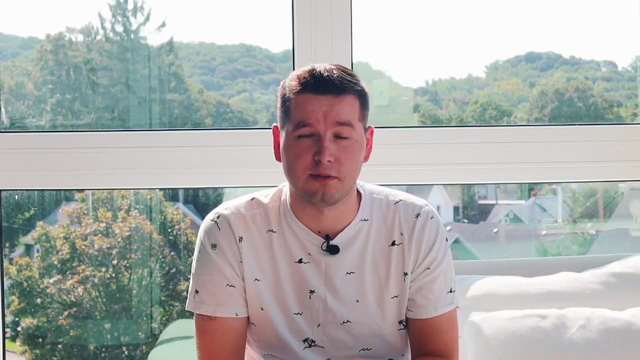 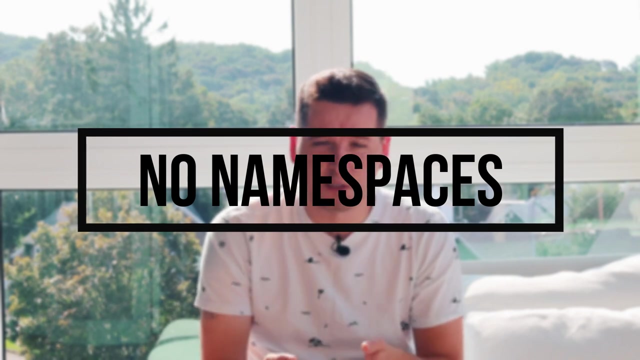 now Seriously subscribe right now. C has no object-oriented programming concepts like abstraction, data hiding, encapsulation and polymorphism. C itself just follows procedural programming approach. That's all it does. C does not implement the concept of namespaces, which means that you can only have one variable named the same way. You can't have multiple variables globally defined with the same name, or even functions. You can't have functions globally with the same name, which makes it kind of annoying sometimes when you write C code Getting out of the C programming. 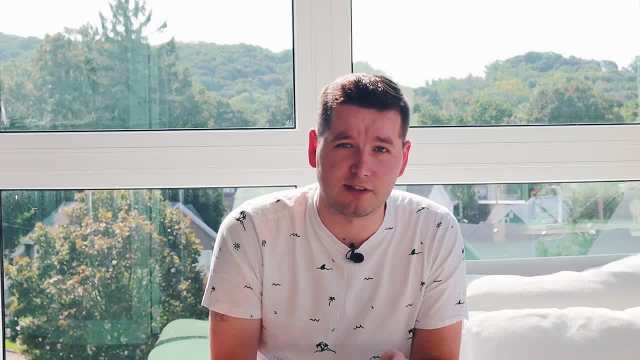 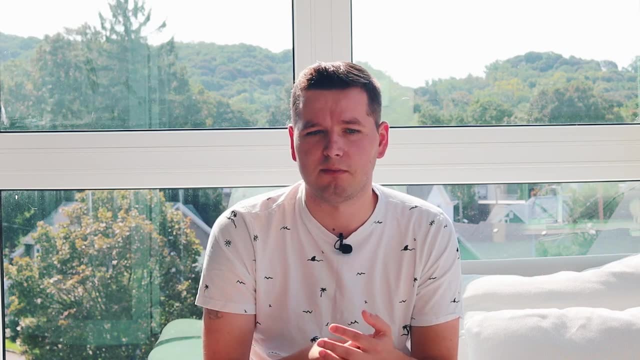 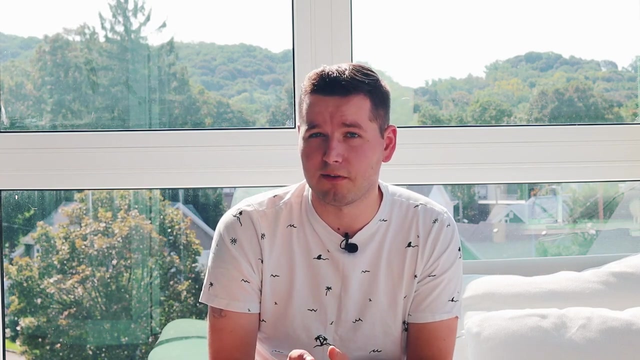 mindset when learning C as your first language can be challenging. When you transition over to C++, for example, it is very common to just be stuck with the mindset that you know I would just keep doing stuff like C in C++ and not utilizing all the cool stuff that C++ offers. I think it's